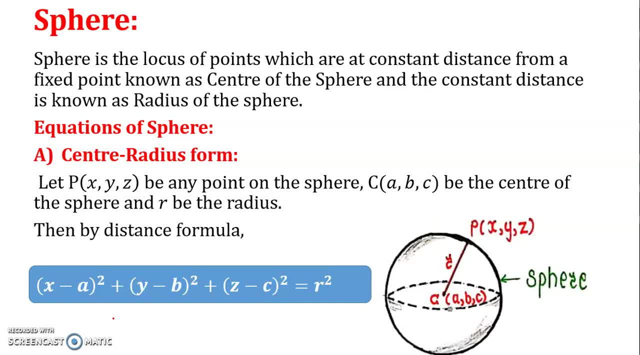 be any point which lies on the sphere along the center a, b, c and radius equal to r. Then by distance formula, if we find distance between the points P and point C, it is square root of x minus a square plus y minus b square. 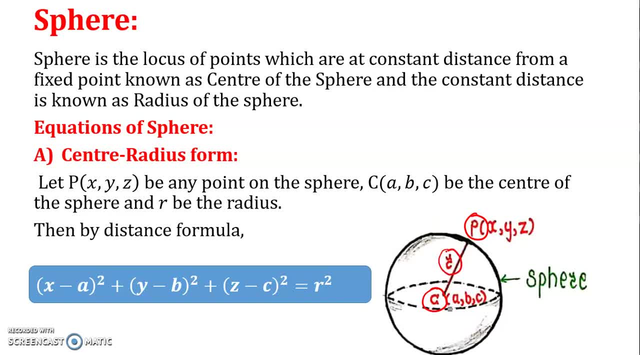 plus z minus c square is equal to r distance between these two points. If you take squares of both sides, we get equation of sphere in center radius form where coordinates a, b, c along x, y, z plus z minus c are given. coordinates for the center and right hand side of the equation will give radius of the sphere. 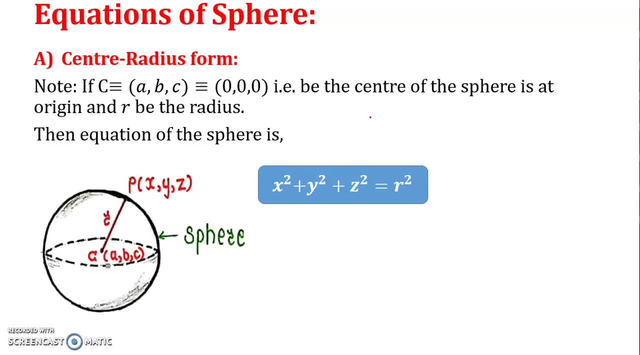 There is specific case if center of sphere lies at origin means if a is equal to zero, b is equal to zero, c is equal to zero. And if we substitute a, b, c equal to 0,, 0, 0, in the equation we get x square plus y square plus z square, equal to r square. 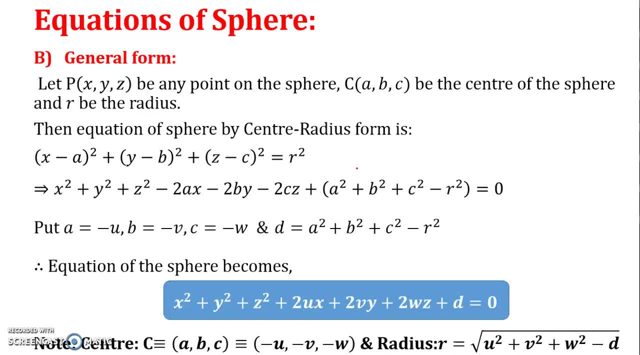 general form of equation of sphere along the center at coordinates a, b, c and radius equal to r can be given by: since our equation of sphere in center radius form is x minus a square plus y minus b square plus z minus c square, equal to r square. if we expand those brackets and simplify, 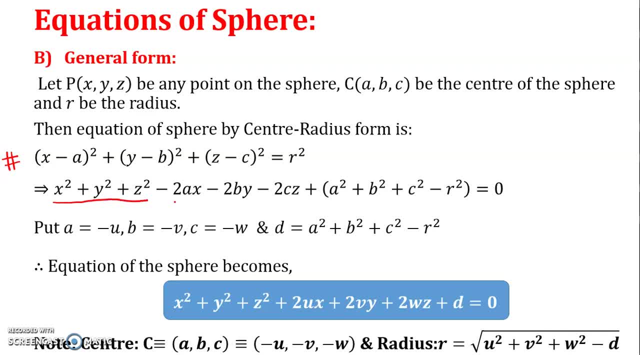 we get x square plus y square plus z square minus 2 times ax minus 2 by minus 2 cz plus a square plus b square plus c square minus r square equal to 0. if we substitute: u is equal to minus a, v is equal to minus b and w is equal to minus c and d is equal to a square plus b square plus c. 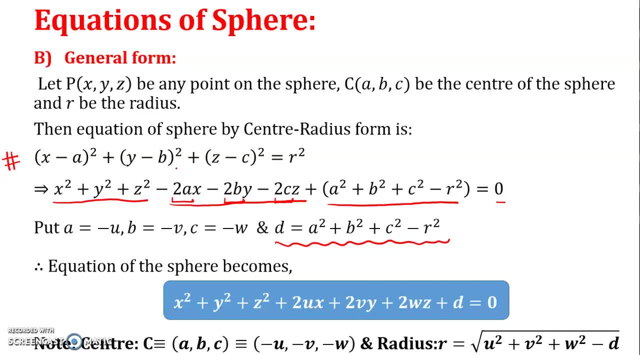 square minus r square, we get the given equation of center radius. form can be written in this way: x square plus y square plus z square plus 2 ux plus 2 vy plus 2 wz plus d equal to 0.. We will refer this as general. 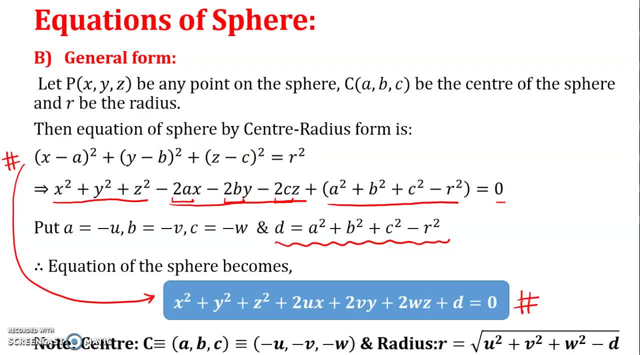 form of equation of sphere, and we will use this as the standard formula, where coordinates for the center of required sphere is minus u, minus v, minus w and radius of the required sphere is square root of u square plus v, square plus w square minus d. Then there is next case. 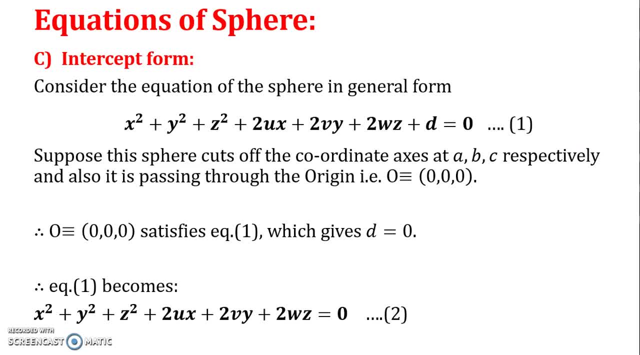 intercept form. if we have a sphere, suppose the required sphere, suppose the required sphere touches the coordinate axis at point a- this is my x axis- it intersects y coordinate at point b, and if it intercepts at point c along z axis, then we call these a, b and c as x, y and z intercepts. 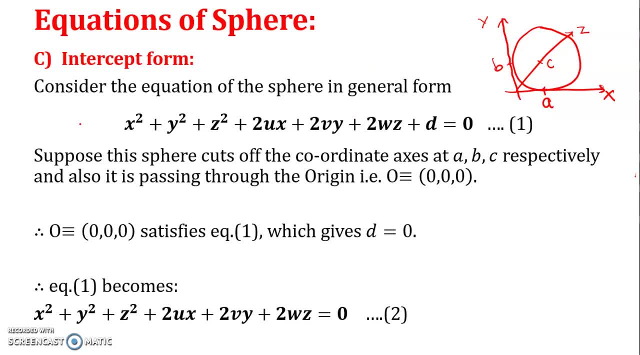 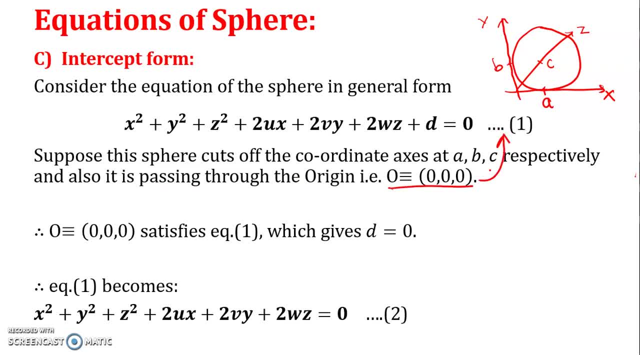 means this will satisfy equation of sphere. so if we substitute x is equal to 0, y is equal to 0, z is equal to 0, we can find required value for d is equal to 0. if we substitute this in equation number 1, our equation will reduce to x square plus y square plus z. 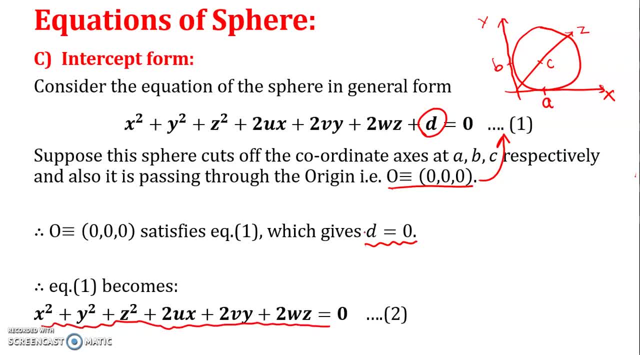 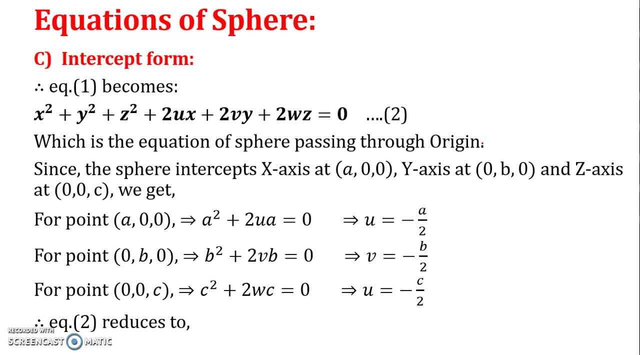 square, plus 2 ux, plus 2 vy, plus 2 wz, equal to 0.. Therefore, since this equation of sphere passes through the points a, 0, 0, 0, b, 0 and 0, 0 c, along x, y and z axis respectively, we can find: 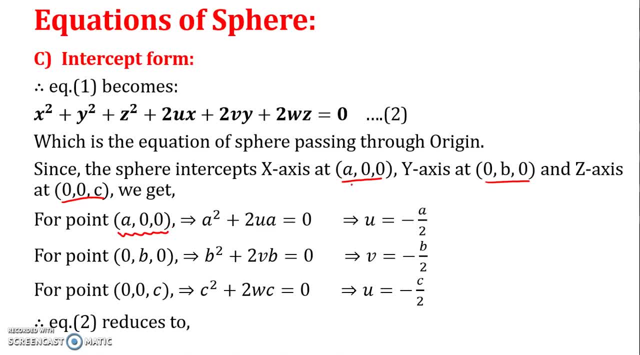 equation of sphere will be satisfied at this point of contact. So at x intercept we find value for u is equal to minus a by 2.. If we substitute, x is equal to 0, y is equal to b, z is equal to 0.. In equation number 2, we find v is equal to minus b by 2.. For 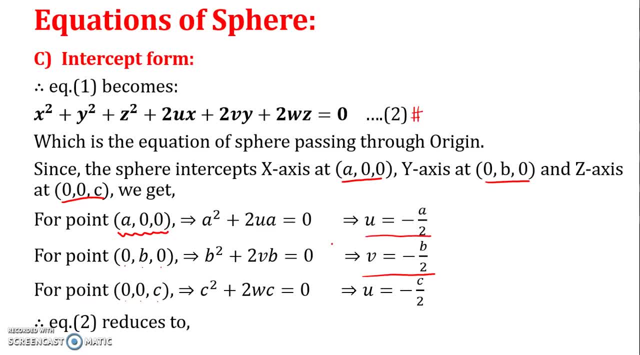 point 0,, 0, c or z intercept equation 2 will reduce to the equation w equal to minus c by 2.. If we substitute the these values of u, v, w in equation number 2, we get x square plus y square plus z square. 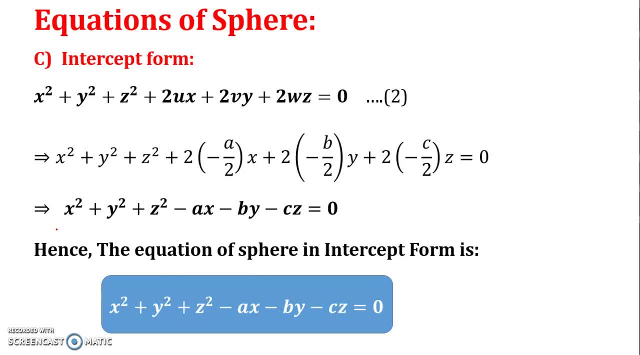 minus ax, minus by minus cz, equal to 0, where a, this a, b and c are x intercepts, y intercept, z intercept respectively. Therefore, required equation of sphere in intercept form. this is, and we will use this as formula: 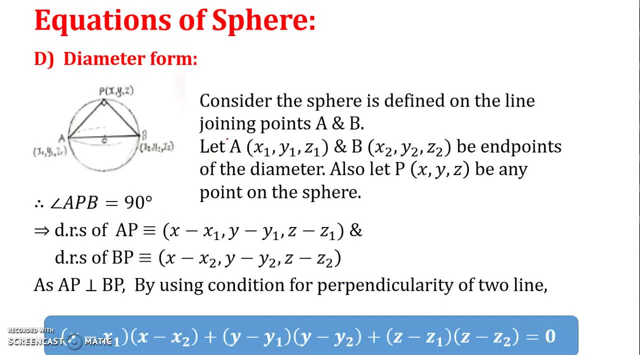 Then next case is diameter form. Consider: sphere is passing through the points a and b, where point a is given by the coordinates x1, y1, z1 and point b is given by x2, y2 and z2.. And the sphere is positive. 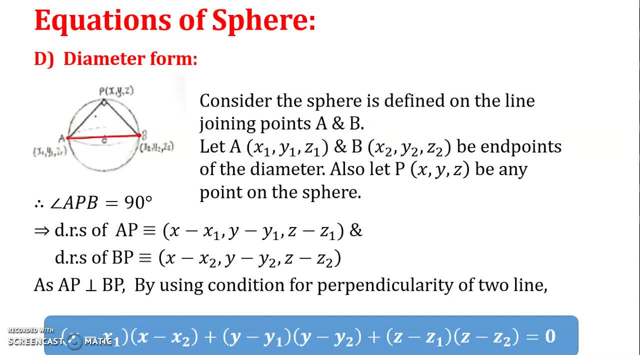 If we consider point p lies on the sphere. these coordinates are x, y, z and this angle, a, b, b- is of 90 degrees. Therefore, direction ratios of line passing through these two points will be: if we consider a line passing through these two points by distance formula, we get: 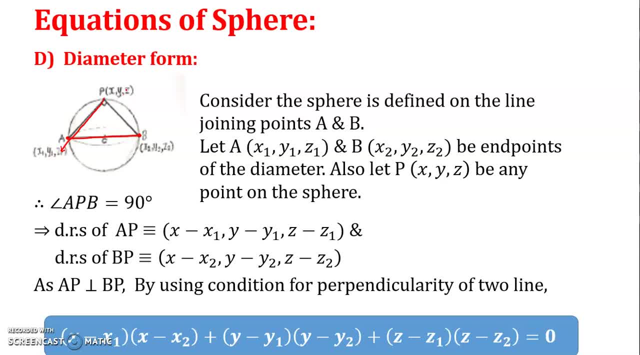 x minus x1, y minus y1, z minus z1.. So these are my direction ratios of line a b. Same is the case with line p b joining these two points. So direction ratios of line p b is equal to x minus x2, y minus y2, z minus z2.. 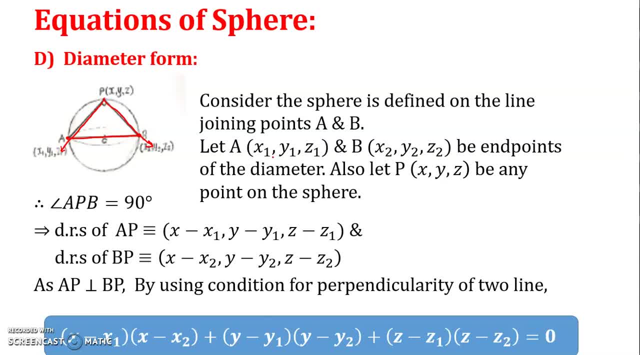 As a b is perpendicular to p b. therefore, by using condition for perpendicularity of two lines, a, b and p b, we have product of direction cosines. let us consider the next example, which will help us determine what we hope to do here. 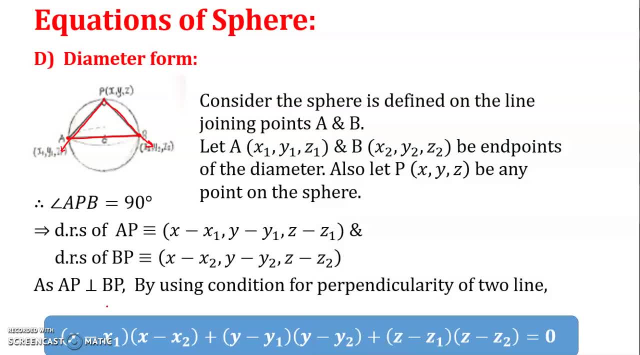 So let us consider a journey of y-1, z-1-2,, because t-x equal to t, has got번 0 to x-1, b-x-1-2,, so we fixed y-x-1 equal to zero. 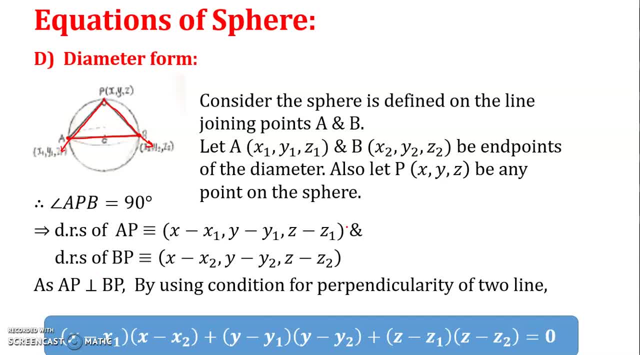 So that is x-x1 plus y-y1, plus z-z1, sorry, x-x1,. x-x2 plus y-y1 into y-y2, plus z-z1 into z-z2, equal to 0.. The last case is if my sphere is passing through 4 points: x2, y1,, 2, interest points d-x-2,. 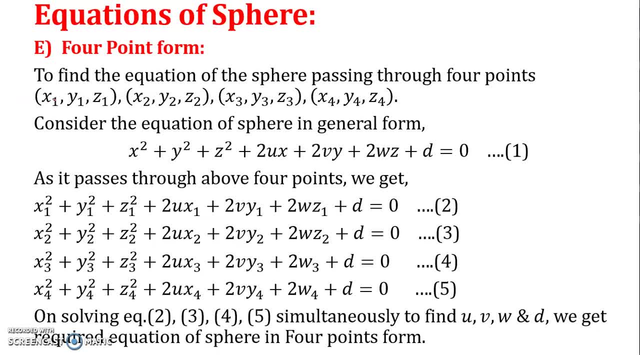 s-2, so we complete the problem. So if I talk length, we take the remaining x for both modes, We will know what they are that are effective to follow points x1, y1, z1, x2, y2, z2, x3, y3, z3 and x4, y4, z4.. Therefore we start with a general. 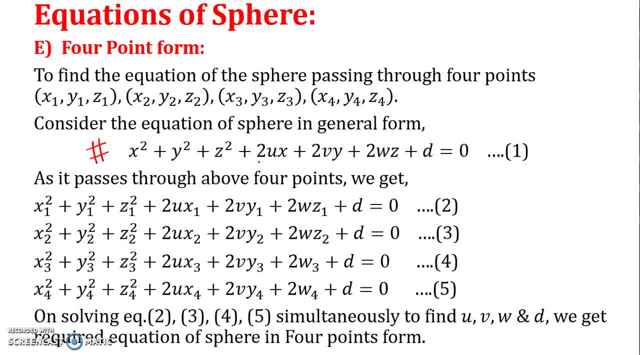 equation of sphere x square plus y square plus z square plus 2 ux plus 2 vy plus 2 wz plus d, equal to 0.. Since the sphere is passing through these four points- x1, y1, z1, x2, y2, z2, x3, y3,- 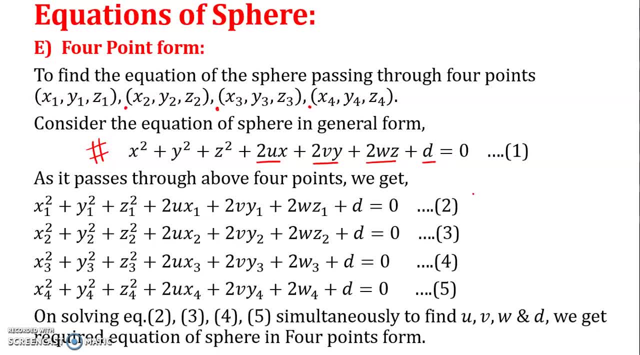 z3, x4, y4, z4, we substitute these values in equation 1.. So we get these four equations in terms of all four points. If we solve these four equations simultaneously to find values for four unknowns- u, b, w and d- we can find the required coefficient and equation 1. 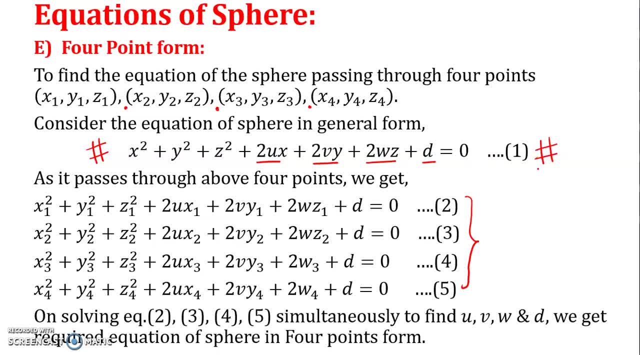 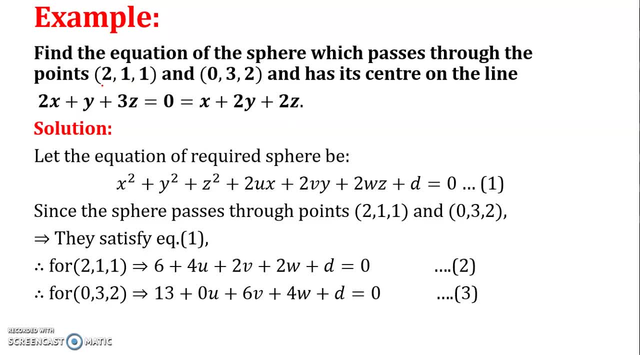 will give the required equation of sphere. So let us take one example: Find equation of sphere which passes through points 2, 1, 1 and 0, 3, 2 and its center lies on the line 2x plus y plus 3z equal to 0, equal to x plus 2y plus 2z. 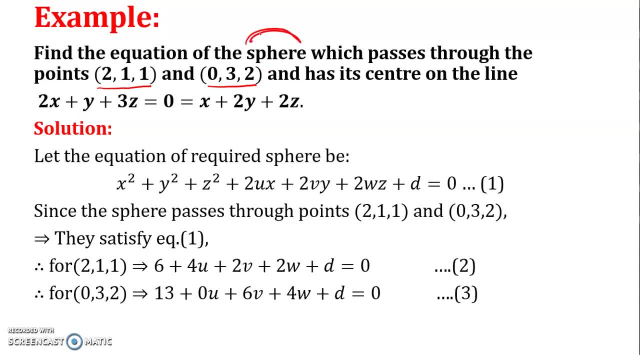 So we have to find equation of sphere. It is not given that sphere is passing through these two points where these two points are passing through, So we have to find equation of sphere. If we join these two points it forms diameter of the sphere. So it is not sure that we are going. 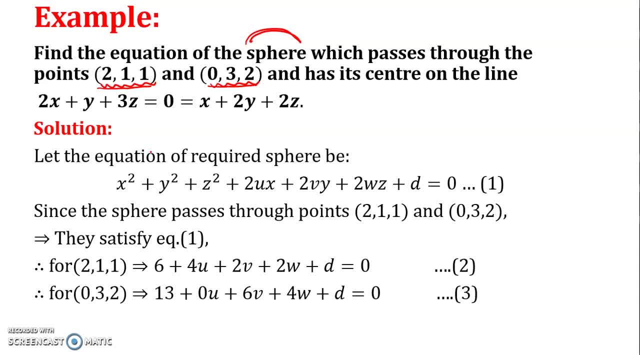 to use diameter form of the sphere. So we start with general equation of sphere. So we consider it x square plus y square plus z square, plus 2ux plus 2vy plus 2wz plus d, equal to 0, be the 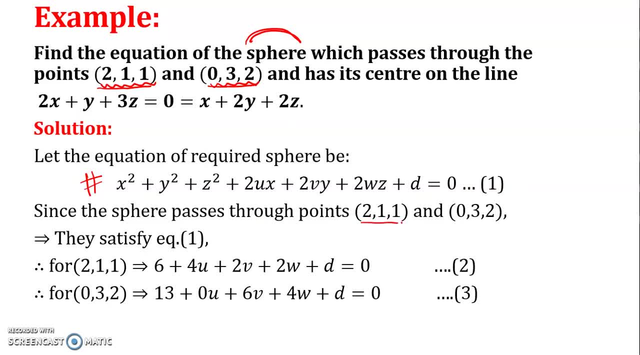 required equation of sphere. Since that sphere passes through points 2, 1, 1 and 0, 3, 2,, it means these two points will satisfy equation number 1.. So, one by one, we find out the equation. 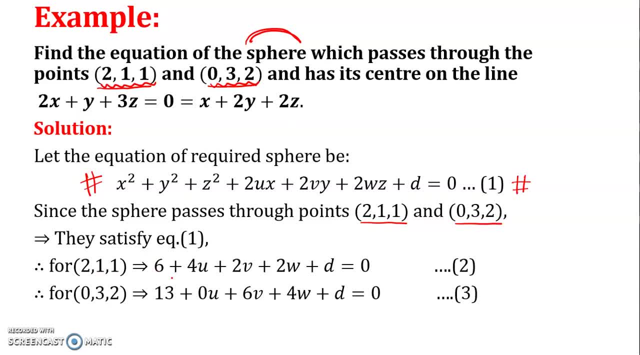 So for point 2, 1, 1, equation 1 reduces to 6 plus 4u plus 2v plus 2w plus d, equal to 0. It is obtained when we put: x is equal to 2, y is equal to 1, z is equal to 1.. Same is the case with 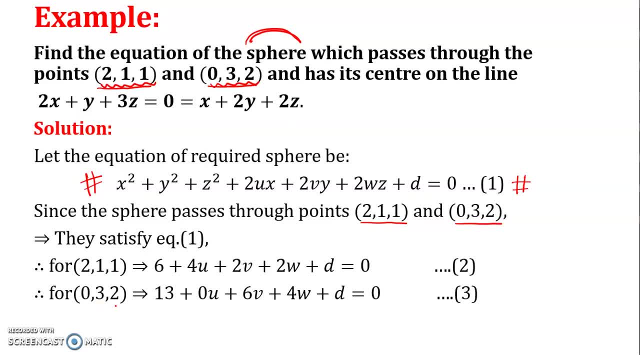 second point: 3, 0,, 3,, 2. We get 0.. So we have to find equation of sphere, So we have to find equation number 3.. So from equation 2 and 3, if we subtract them together, if we subtract, we find an. 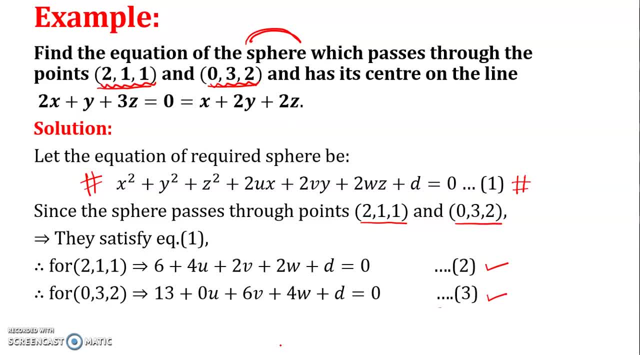 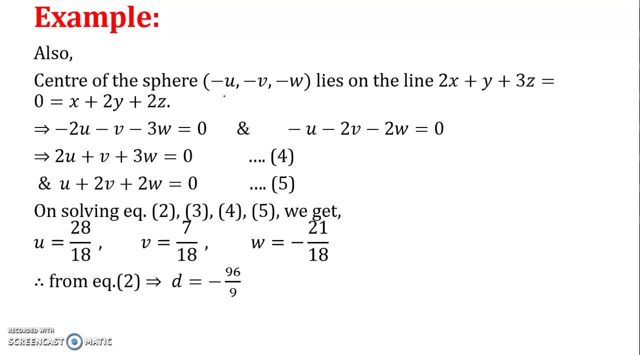 equation in terms of variables u, v and w only, So that we eliminate variable d, Since center of the sphere, that is, minus u, minus v, minus w, lies on the line 2x plus y plus 3z, equal to 0 and x. 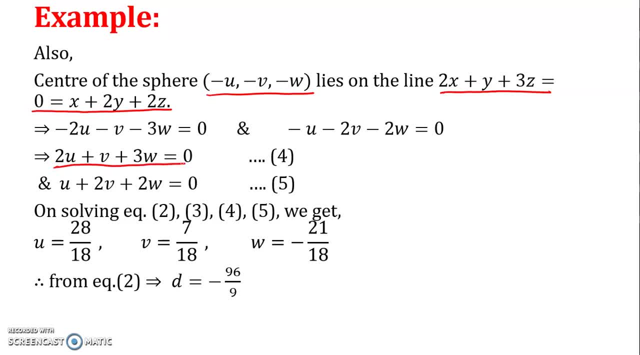 plus y plus y is equal to 0.. So we get the two equations 2u plus v plus 3w, equal to 0.. u plus 2v plus 2w, equal to 0.. So therefore, from equation 2,, 3,, 4 and 5, we get, Since we eliminate variable, 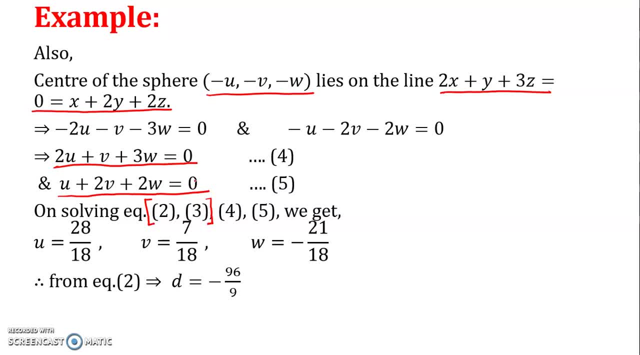 d. from equations 2 and 3, we retrieve an equation containing variables u, v, w. So this will give an equation. Equation number 4 and equation number 5 will give us a system of linear equations Containing variables u, v and w. We can apply matrices method to simplify that system, or we can. 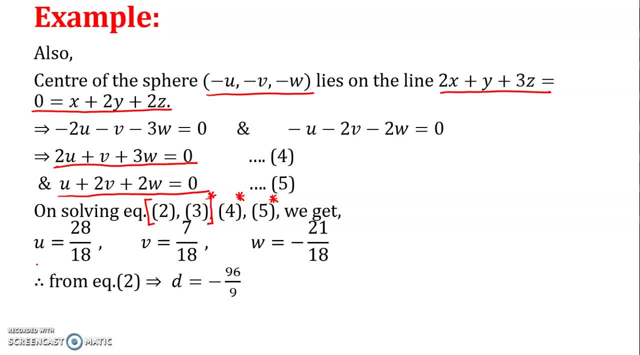 use Cramer's rule to find values for u, v and w. So therefore, if we solve that system, we find u is equal to 28 by 18, v is equal to 7 by 18, w is equal to minus 21 by 18.. If we substitute: 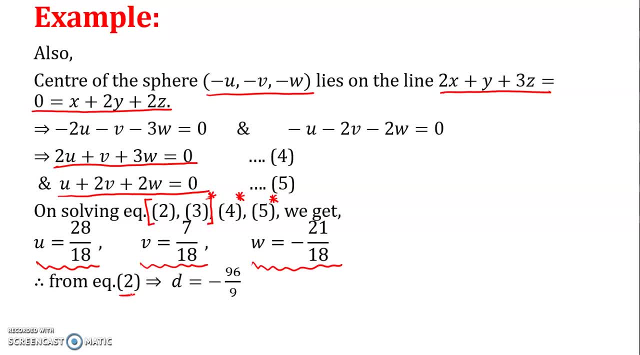 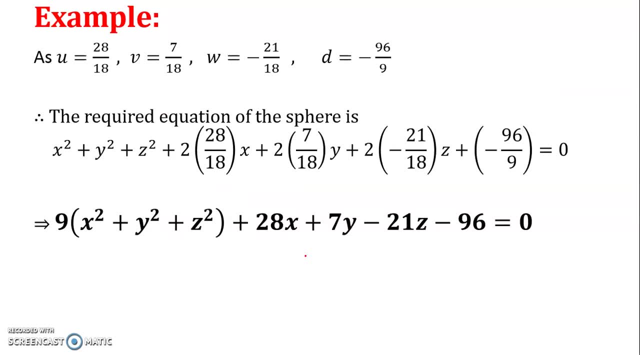 these values of u, v and w in equation number 2, we can find: value for d is equal to minus 96 by 9.. So, as we obtain all the unknowns for given equation of sphere, u is equal to 28 by 18, v is equal to 7 by 18, w is equal. 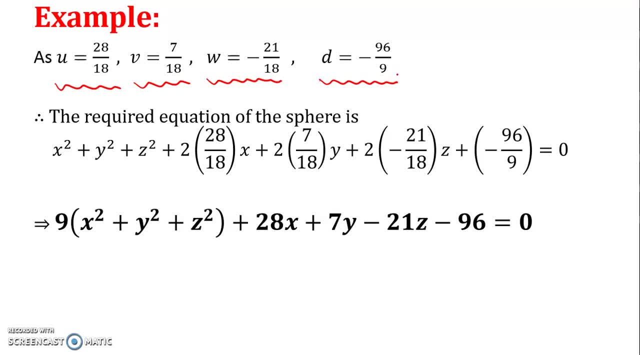 to minus 21 by 18, and d is equal to minus 96 by 9.. Therefore required equation of sphere in equation number 1 will reduce to. So we substitute value for u, v and w. So this is the equation. 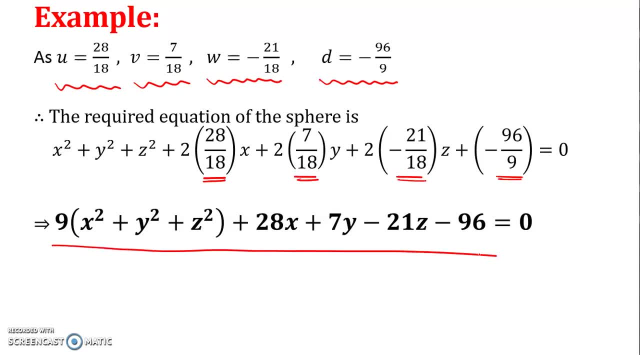 W and D, So this will be the required equation of sphere. Here, while solving examples, we have to take care of the given data. If it is clearly or specifically mentioned that these two points forms diameter of the required sphere, then, and then only, we will use diameter form of equation. 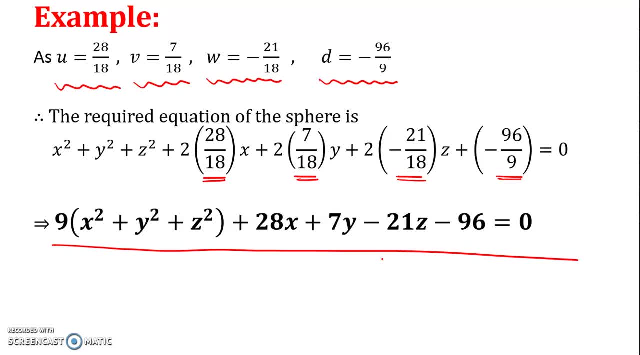 of sphere. Otherwise, we will start our solution with a general form, and in general form of equation of sphere, we need to identify values for U, V, W and D. Thank you.